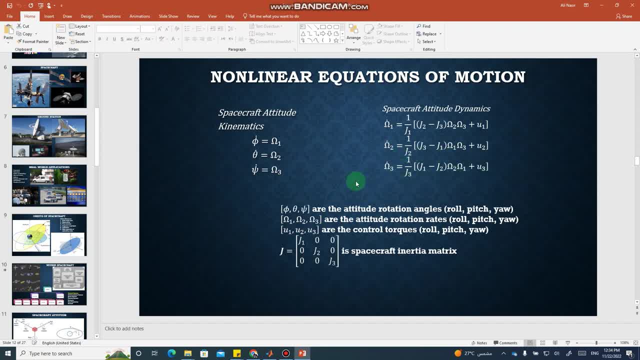 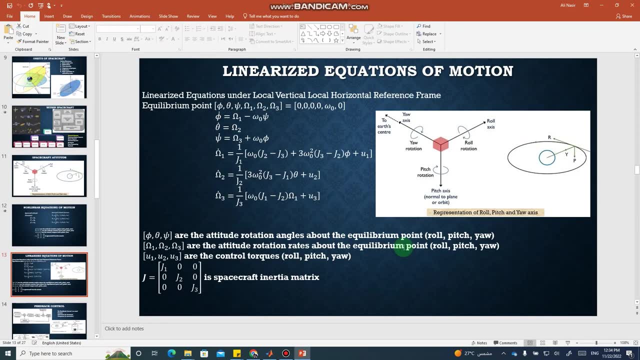 pitch axis and u3 is the torque vector along the y-axis. so we need to see how to make MATLAB simulations of these equations and how to design the controller. we will get back to this in a moment. just before that, i just want to show you some linear equations of motion as well. so these 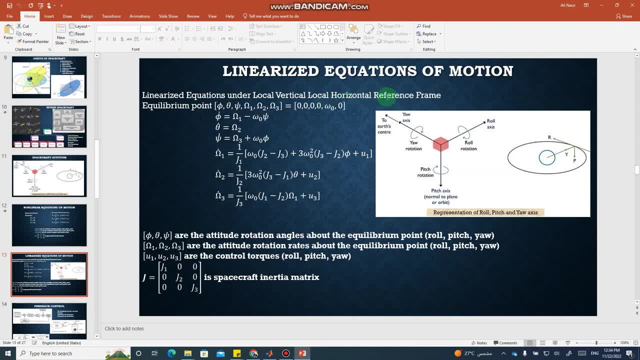 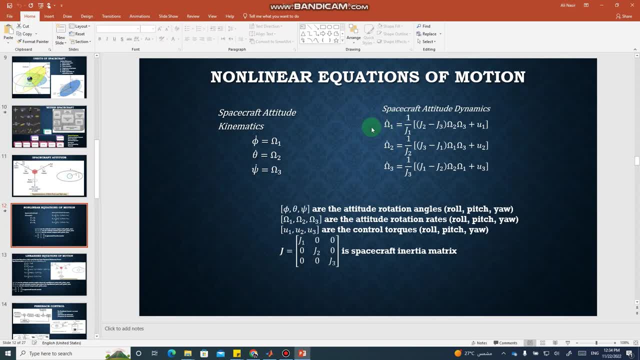 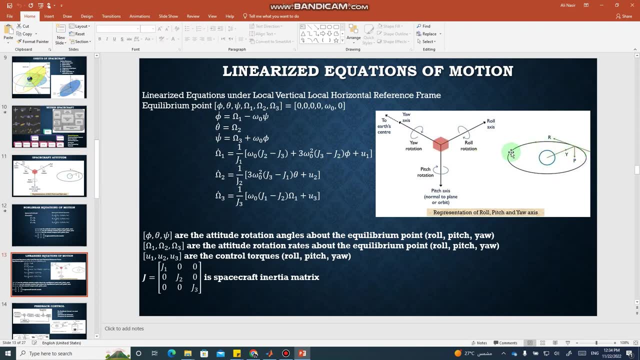 are the equations of motion under local vertical and local horizontal reference frame. so these are the non-linear equations. are with respect to body, fixed frame, but here this frame is also fixed with the body of the spacecraft. but the difference is that this frame is a rotating frame. so this frame is rotating along with the 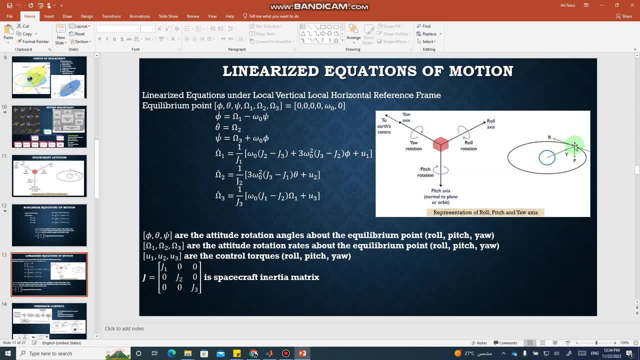 spacecraft, and this is useful for the spacecraft which are which have like communication antenna which has to point continuously towards the earth. so for this type of spacecraft these linearized equations of motion are are very useful. so here, roll roll angle rate is not just omega 1, it is. 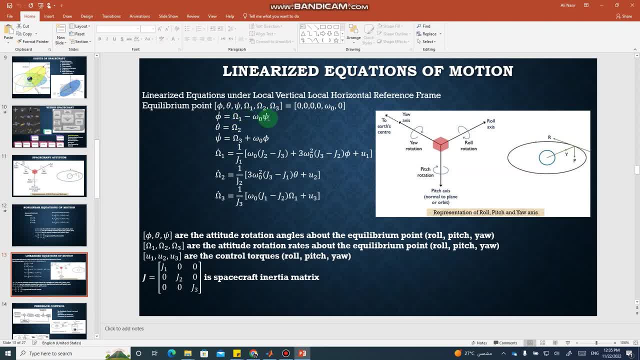 omega 2 and omega 3. so this is the linearized equation of motion, and this is the linearized equation of motion. and this is the linearized equation of motion, and this is the linearized equation of motion minus this omega naught times psi, which is yaw. this is because this is the rate of rotation in this. 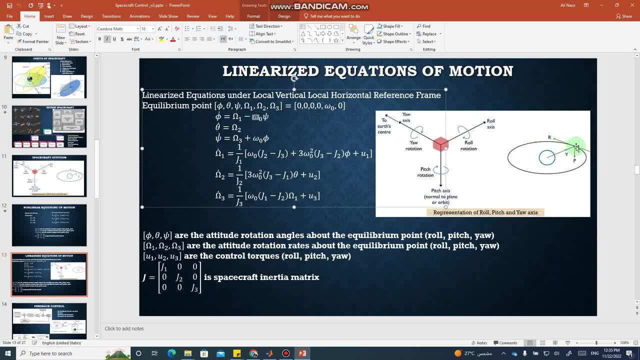 orbit like the. imagine a spacecraft which is one face of the spacecraft or an antenna of the spacecraft, is continuously pointing towards the earth. as the spacecraft goes around the orbit, it will be rotating like it. in order to keep the antenna continuously pointed towards the earth, the spacecraft will have to continuously. 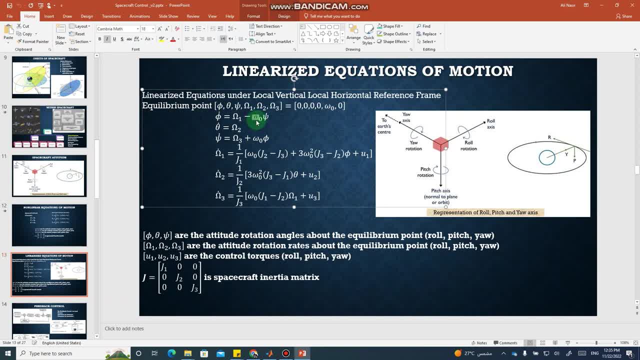 rotate at an angle at a rate of Omega, naught this Omega 0. so then theta dot is equal to Omega 2, and then psi dot is equal to Omega 3 plus Omega naught into Phi, then Omega 1 dot is equal to the same similar equations as we saw in the 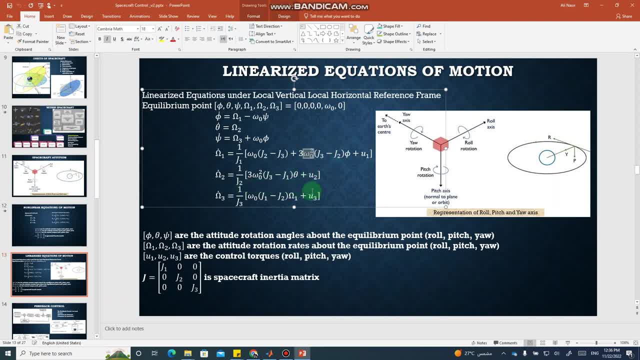 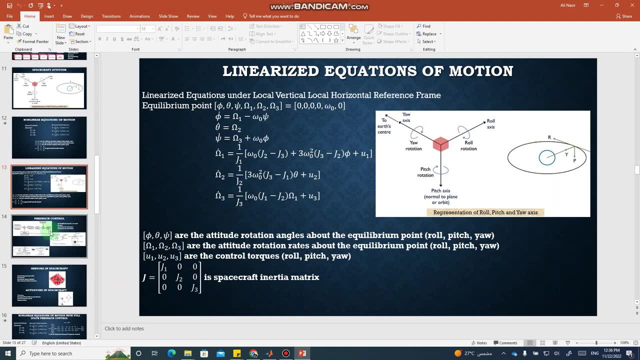 previous slide, but there are some terms involving the rate of rotation of the orbit LV LH, the local vertical, local horizontal orbit, and then we will simulate these equations of motion as well and then we will also design the feedback control. so feedback control are of different types for spacecraft and 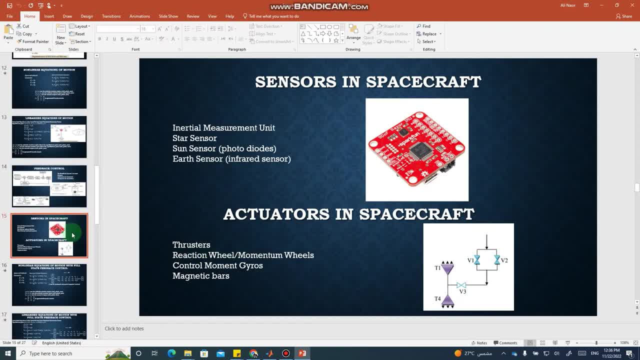 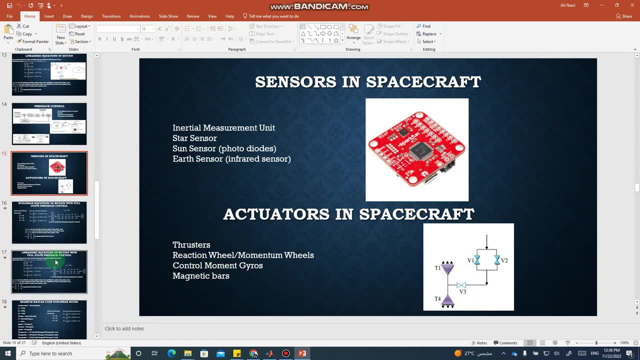 there are different sensors and actuators that are used in the spacecraft as well, like inertial measurement unit, star sensor, Sun sensor, earth sensor and reaction. we'll control motion and then we will also design the feedback control, and there are different sensors that are used in the spacecraft and there are different sensors, so 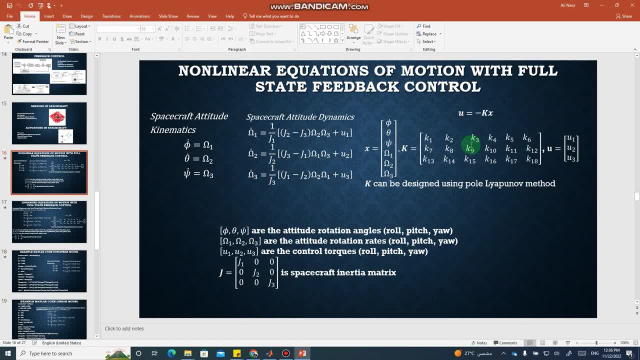 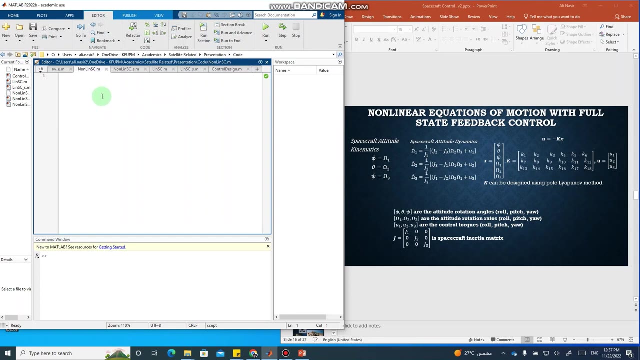 and the same controller will work for the no linear model as well. so we will see how the controller is designed and we will also see how the equations of uh start from here and here. this is matlab, so i will just create a function file in matlab. so function: non-linear spacecraft dynamics, and here first i have to specify the 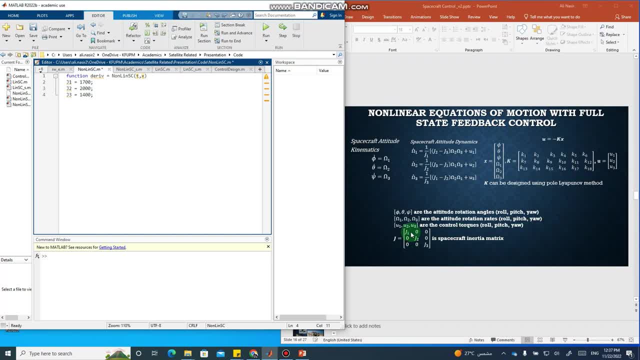 the inertia values, so these will depend on the size of the spacecraft. i have just taken these values out of some textbook. so this is like j1, j2, j3- the inertia across different axes. this is like a year of how big the spacecraft is. then i define omega like omega 1, omega 2, omega 3. 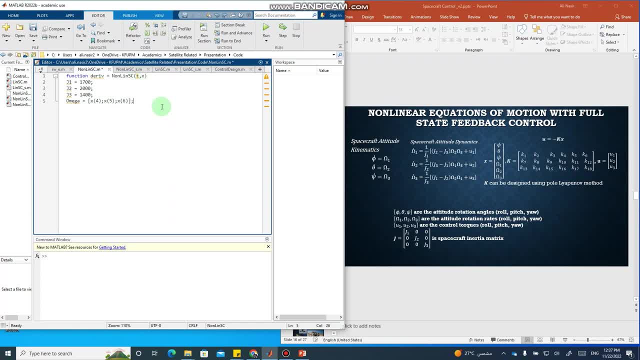 to be the fourth, fifth and sixth part of the state space, and then controller design. we will come to this in a little bit that i designed the controller using pole placement here and we will see how this is done. so u is equal to minus k, x. then phi, dot is equal to omega. 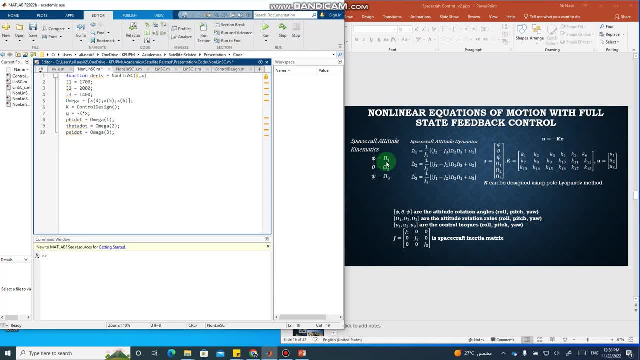 1. then phi theta dot is equal to omega 2, psi dot is equal to omega 3, omega 1 dot. this, this whole equation, and then we have omega 2 dot, omega 3 dot, and in the end we return all of the six derivatives of the states in the 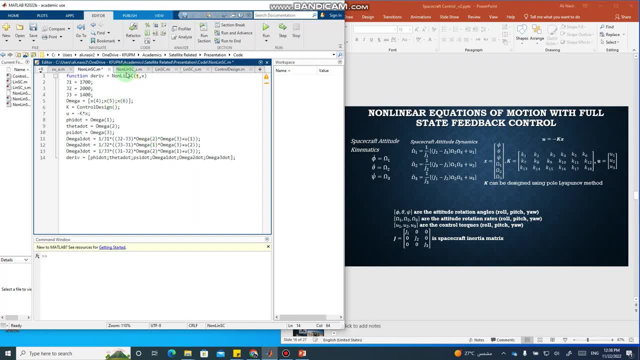 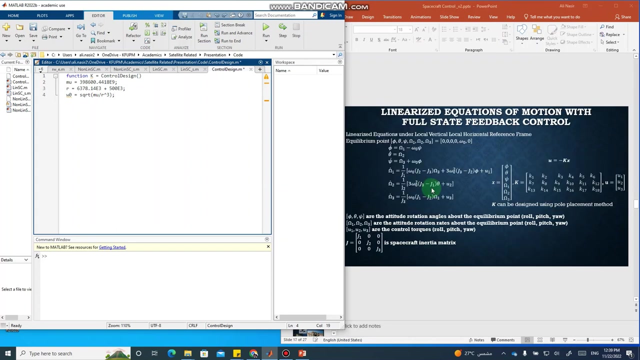 in our function. so and then we have to like design the controller. so, in order to make the controller, i am just designing this control design function and this for this i am using this mu r and omega naught, because this controller was basically designed for this type of this type of equations where there is omega naught. so, since this controller works for 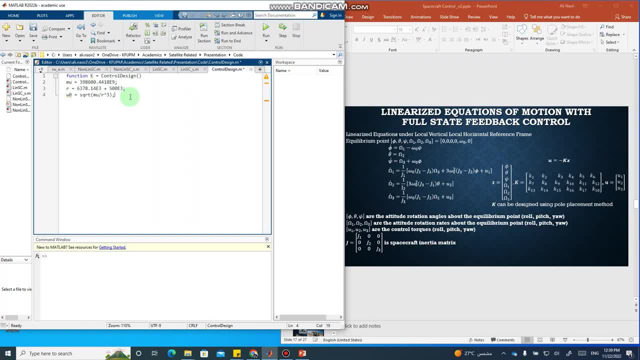 both type of models. so that is why i am including these values and this is just a, just a gravitational constant, and this is the radius of the earth. and then i have the, the inertia of the spacecraft, some a1, a2, a3, because i need to convert this whole equation. 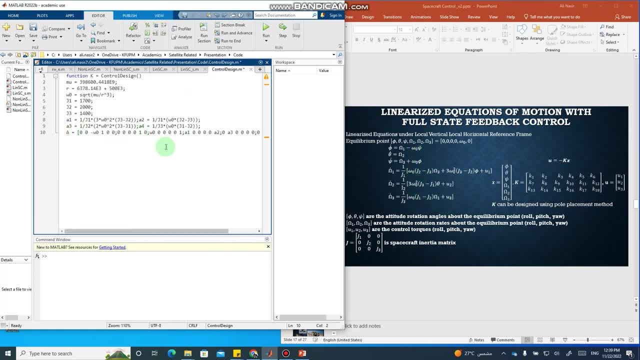 into matrix form. so i create the a matrix and then i also have the b matrix and then i use the, the place command for the control design. so i i don't have to use this as a function in this file. uh, what i can do is i can just calculate the k from here one time and just copy the value of k into this. 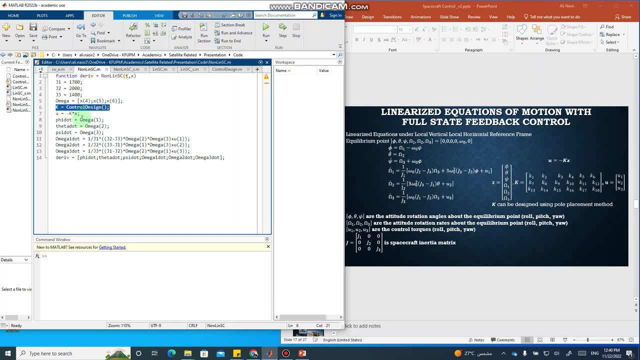 this file into into into this file. so instead of calling the function in this within a function. this is not the the best approach. so once i have this controller design done, then i can just go here and use the ode45 function in matlab and this function will. i'm just giving some initial angles and initial angular rates and 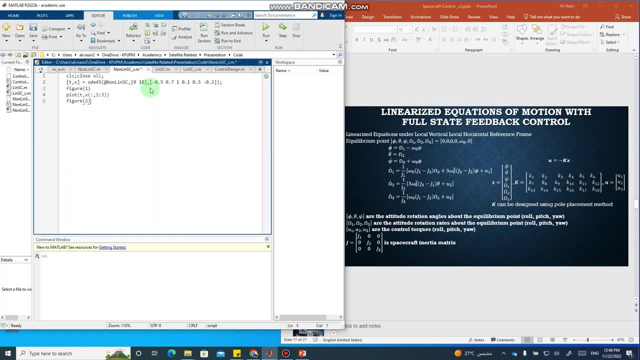 i'm running this simulation for 10 seconds and here i can plot the angles in figure 1 and angular rates in figure two. um and notice this in the controller design. in the pole placement i have placed the poles of the glow loop system at minus one minus two, minus three, minus four minus five and minus. 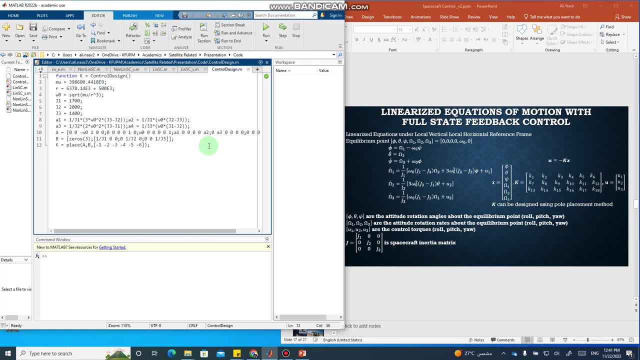 six. you can basically place the poles anywhere you want and you can also place the poles according to the requirements of settling time, rise time and overshoot that you have in your project. so once we have this- the non-linear equations- done and this script file done and we have this controller design done, then we can just run this file and this will give us the 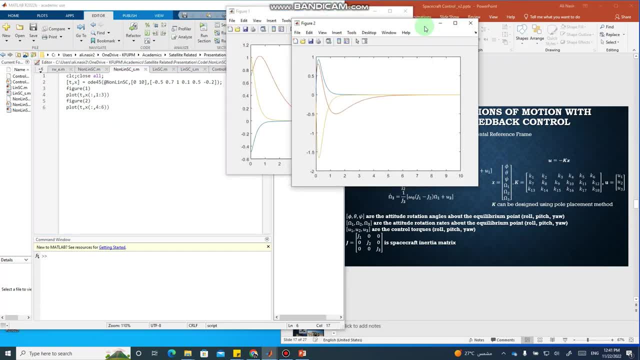 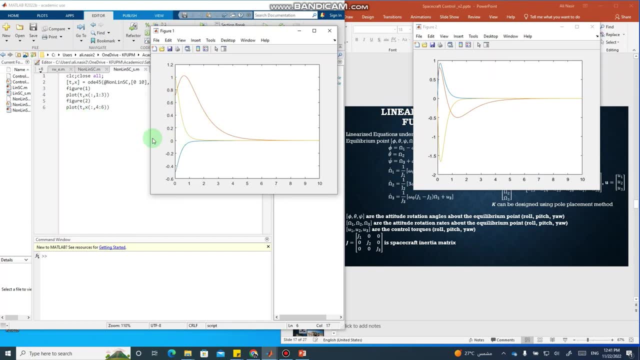 plots of the angular rates and the. so figure two is the plot of angular rates and these are the plots of angles. notice this: i have not put the grid on, or x label, y label. you can see that i have not put the grid on, or x label, y label. 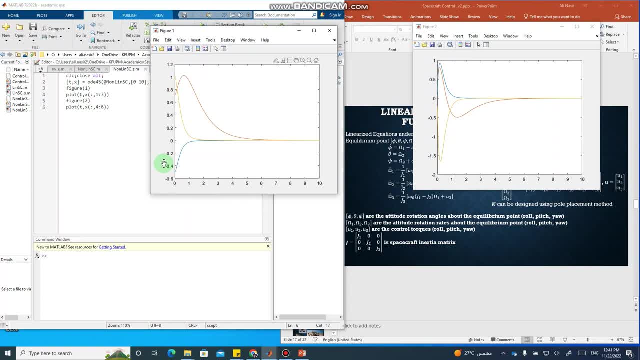 because this just you can get how to put x label, y label and how to make your plot more readable through matlab tutorials on youtube. and here you can see that the initial angles angles were initially not at zero, so the controller is able to stabilize the angles within seven seconds and similarly, the velocities have been stabilized to zero. 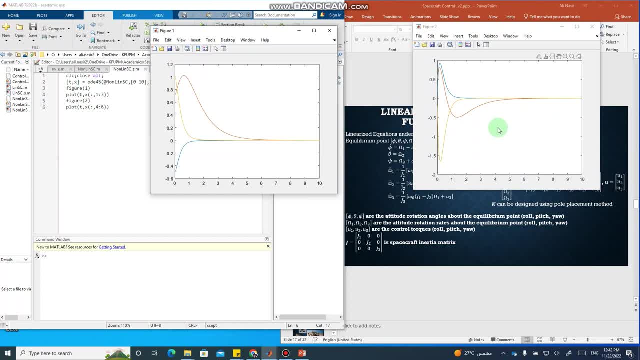 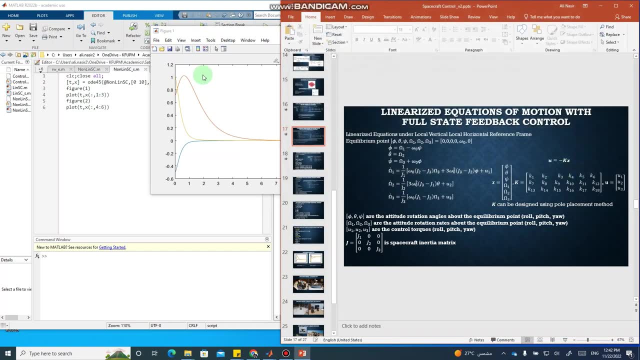 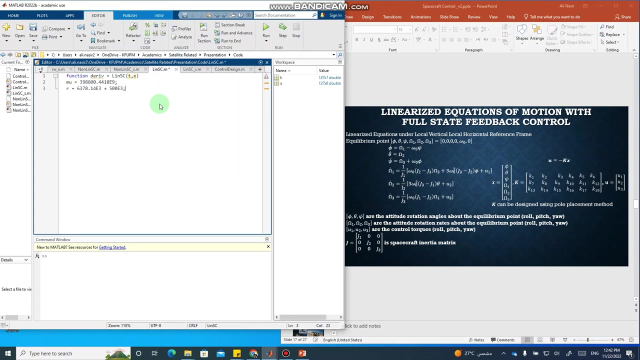 so this next we look at the we, we look at the linear part of the equations. like these equations and these equations we can just simulate or create a function in the linear spacecraft dynamics. here we need the mu and r and omega naught, and these are the inner. 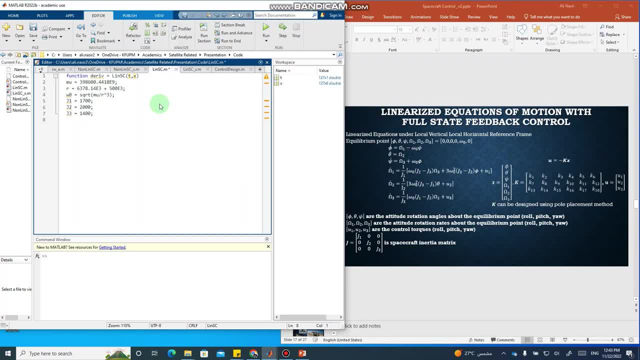 0, обычно mushunya- values of, uh say, spacecraft along different axes. this is control design, same function as we defined. like here again, we don't have to define the whole function because we just calculate the value of k one time and just copy the value in. 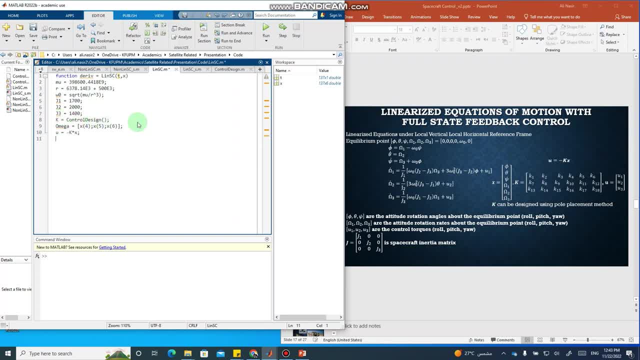 here, instead of calling the function and then use equal to minus x p dot. this is the, this equation, this theta dot. omega 2, all of these equations. i will just write them down: omega 1 dot. omega 2 dot. omega 3 dot. these are the same equations that are written here and then you can just complete.